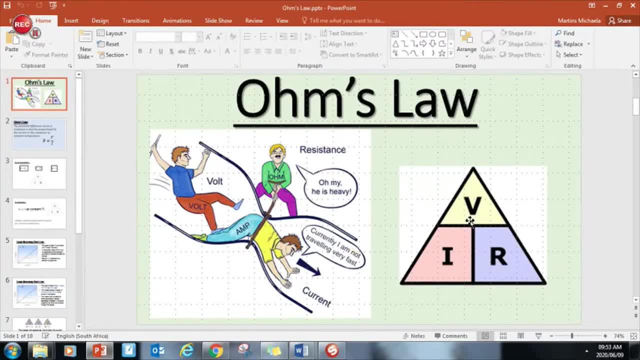 resistance. So this little triangle comes into play. over here We're going to be speaking about the mathematical relationship between these three things. Here's a little photo again, just to illustrate what these three things are and what they do. So the voltage or potential difference. 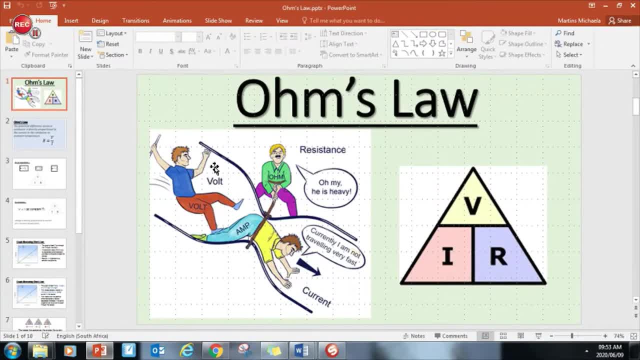 gives the push to the current, to the little charges in the circuit. So you see he's kicking the amp. So that's the current, The current flows and the resistance resists the current, So it kind of impedes the flow. So yeah, you can see he's tying a little rope around the current and this current. 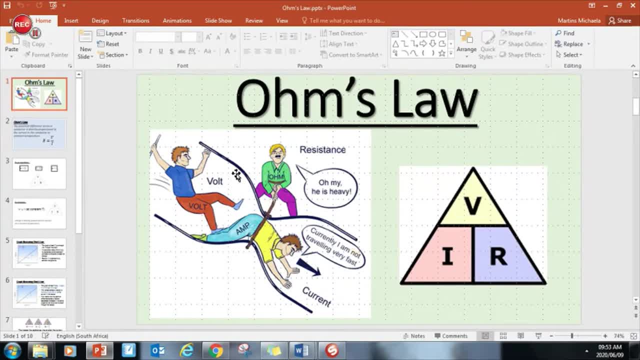 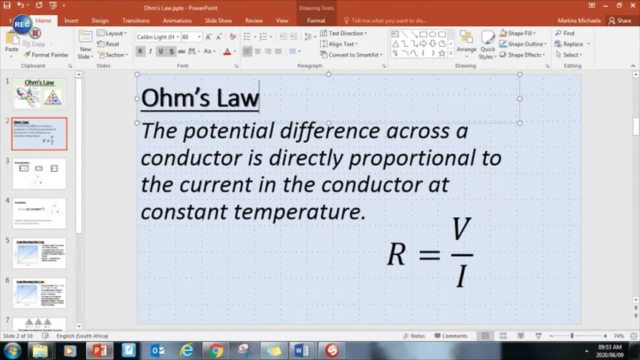 guy is saying: currently I'm not traveling very fast. Okay, it's supposed to be funny. Okay, Ohm's law, This is a definition that we can ask you, So maybe I should just make that clear definition. I'll write here and I want this in your books, please, because this is the number one new definition. 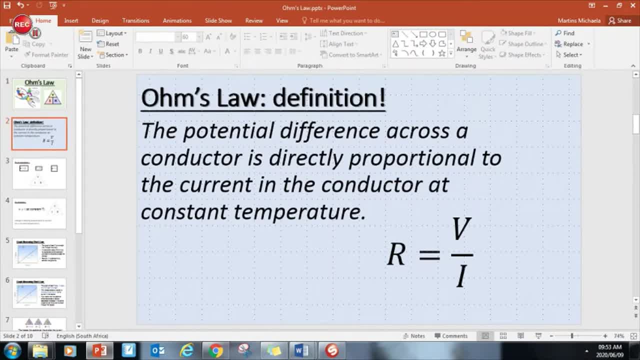 you're learning this year in grade 11.. So let's read: the potential difference across a conductor is directly proportional to the current in the conductor at a constant temperature. So it's this: v equals i times r thing. So potential difference is directly proportional. 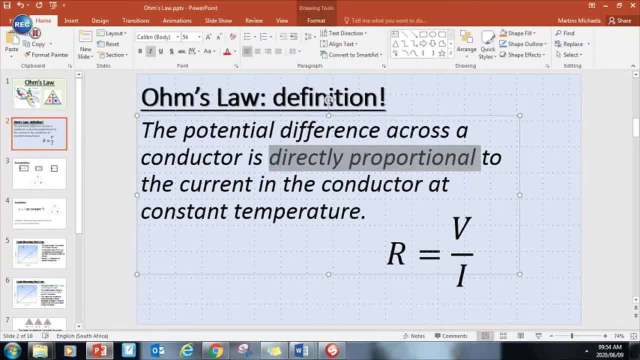 to current, and you know what directly proportional means. Here we go with the mathematical relationships. okay, so it means that as the one goes up, the other one goes up by the same amount. in the same proportion the one goes down, the other one will go down, so as potential difference or voltage. 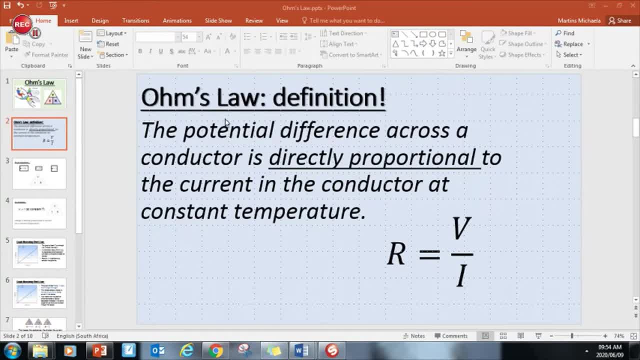 increases, so will the current increase. and that makes sense because, remember, the potential difference is the push that the charges need and when we push the charges, that causes current. so if we give more push, okay, that sounds weird. if we provide the charges with more of a push, so more. 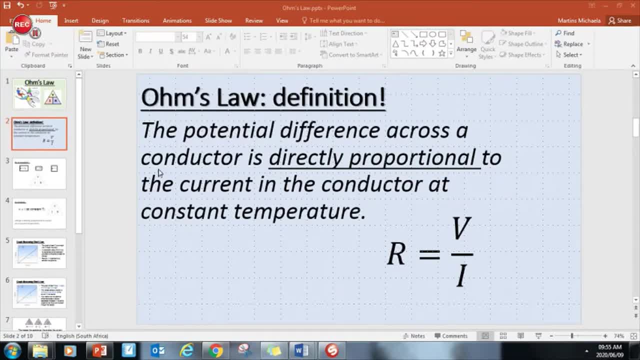 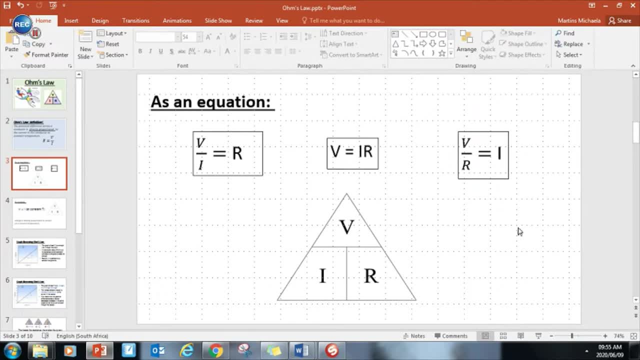 power. basically, essentially, then we'll have a stronger current. okay, here's the relationships. again, we can use this triangle to derive any one of the three equations. it's the same thing. it's just isolating a different variable each time, and okay, so this is ohm's law as an equation. 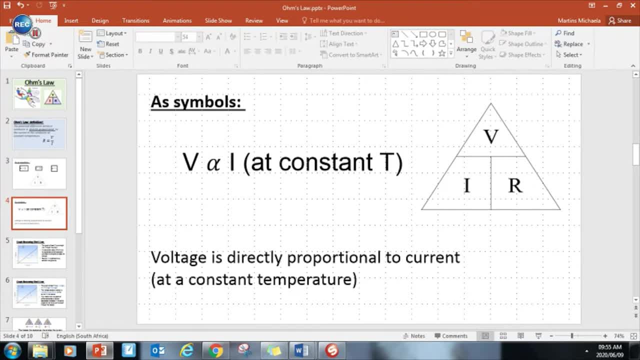 over there and this is ohm's law as symbols. so v, voltage or potential difference is directly proportional. that's a little fish sign to i which is current, but the thing is it must be at a constant temperature temperature. If we change the temperature this relationship will not work. So voltage is directly. 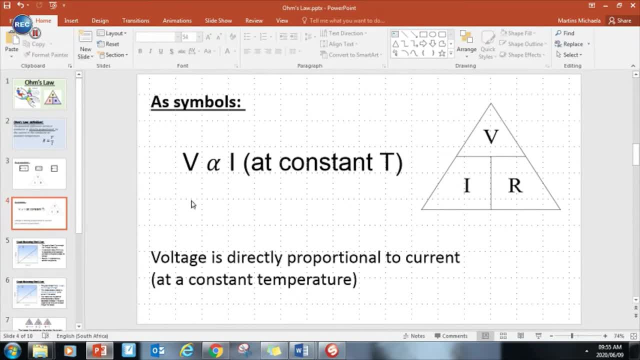 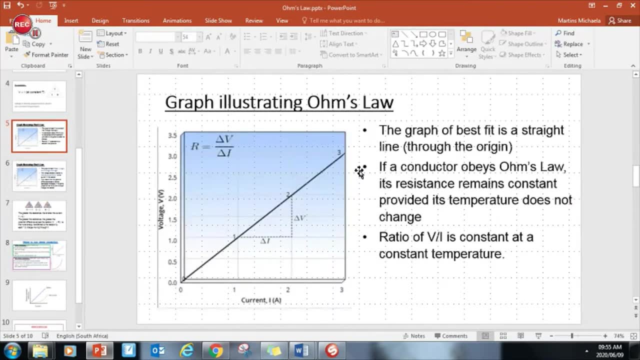 proportional to current at a constant temperature. This is important and you need to have that in your book as well. Okay, now we have a graph. You can potentially receive a graph like this in your exams and you have to understand what's going on. So over here we have voltage on the y-axis. 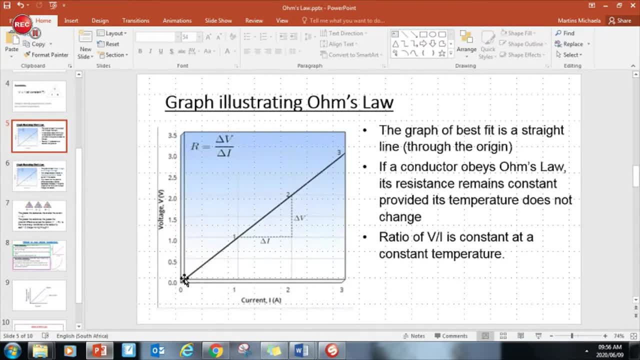 current on the x-axis and we have a straight line, a graph that's a straight line going through the origin. In other words, it cuts at zero, zero. So here it says the graph of best fit is a straight line through the origin. That's important, And what this means is if it's a straight line and 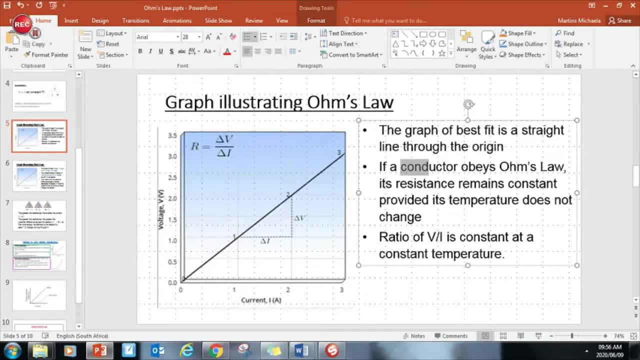 it's going through the origin. it means that the conductor is obeying Ohm's law, And Ohm's law basically says that the resistance will remain Constance provided that the temperature doesn't change. So if you look here, voltage divided by: 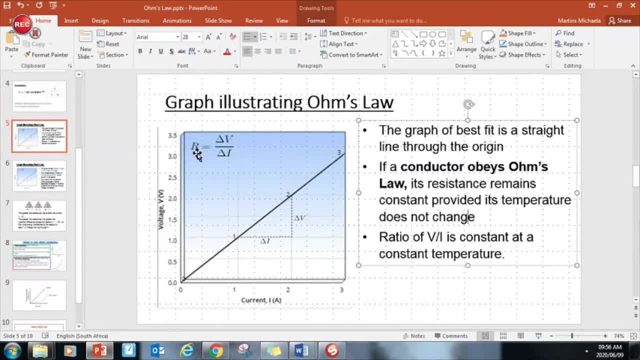 current will give you resistance and the resistance won't change. So as I go up in voltage I'm going to go up in current by the same proportion, So this ratio won't change. So say, for example, it's 10 divided by two will give you five, or 15 divided by three will give you five, or 50 divided. 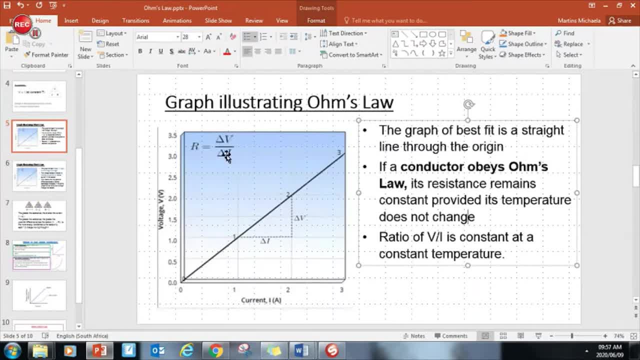 by 10 will give you five. So you can see that the ratio of voltage and current will give you a constant R And that's why the graph is straight and it goes through the origin. You can think of this line, this, the gradient of this line, as being resistance, because we know that we calculate. 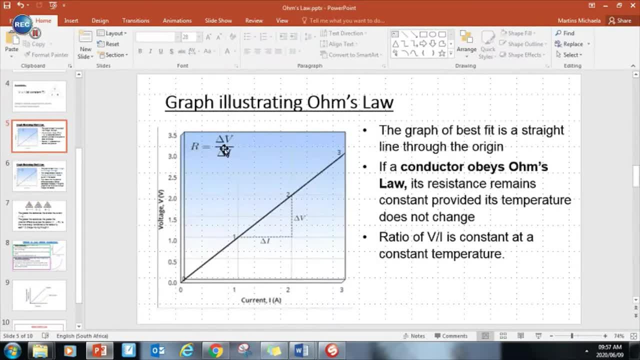 gradients. You should know this. This is literally grade nine work. We calculate gradient by saying the change in Y over the change in X. So what is Y on this line, On this graph? my Y is my voltage. So change in voltage over change in currents, change in X, That. 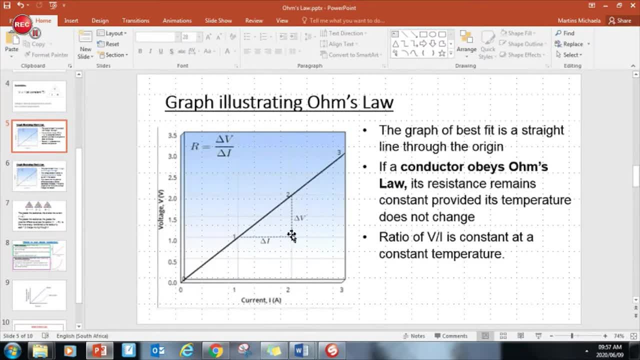 gives my gradients. Yeah, they give you the little triangle. We know that that is used to illustrate gradients: change in Y over, change in X or rise over run. However you learn gradients or learned gradient, that will give you the gradient of the line, which is resistance, And you can see the 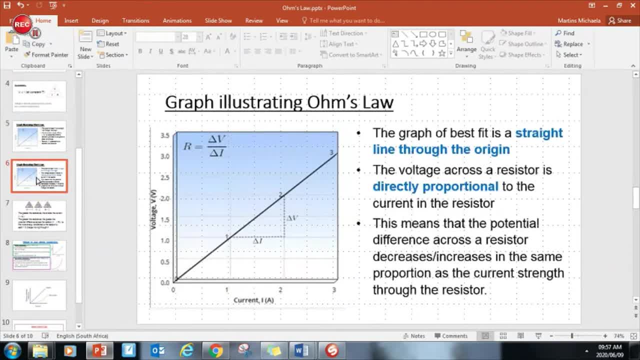 gradient stays constant. cap. Another thing just to note again: the best Fits straight line through the origin. That means that voltage is directly proportional to the current. So as voltage increases, so does current by the same proportion, yet is in the same. 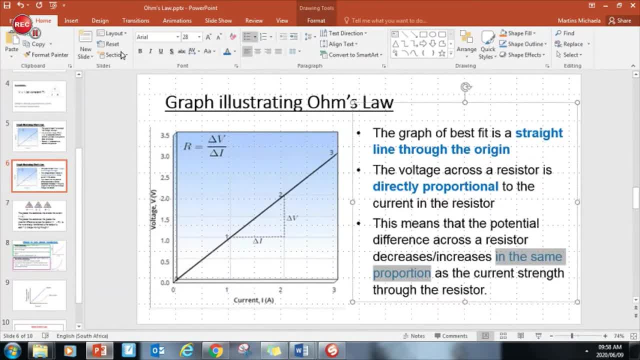 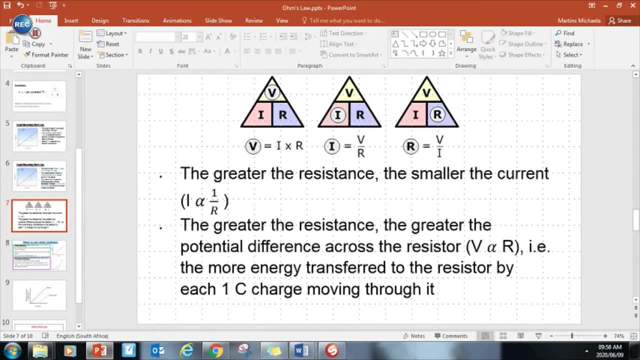 proportion. So we know that that is what that mathematical relationship means. Okay, so let's just take a look at these formulae. I'm saying here, the greater the resistance, the smaller the current. So look at this middle formula here. If I make our bigger, so resistance bigger. 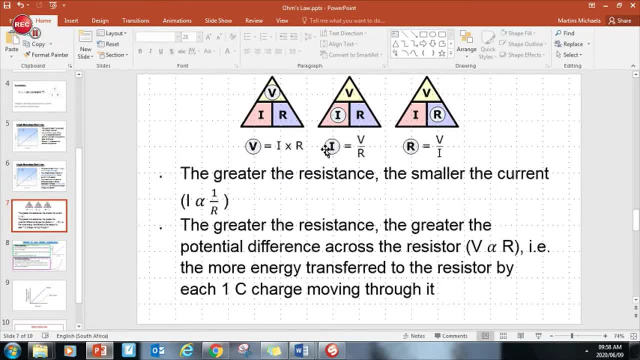 smallest, So big number. I is going to go smaller. So the greater the resistance, the smaller the current. So in terms of the mathematical relationship it makes sense. But also think of it logically. So if I'm providing a greater resistance, so I'm resisting the flow. 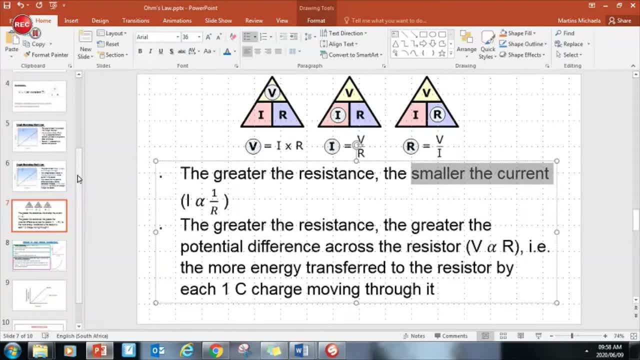 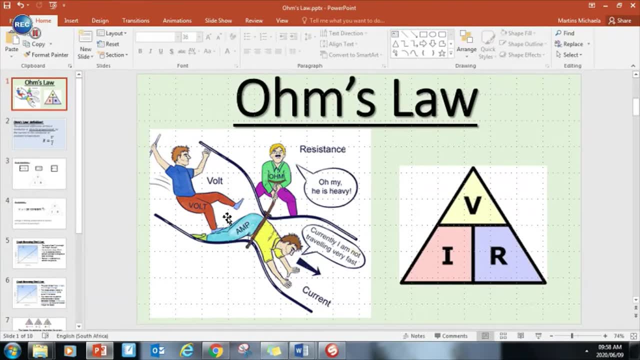 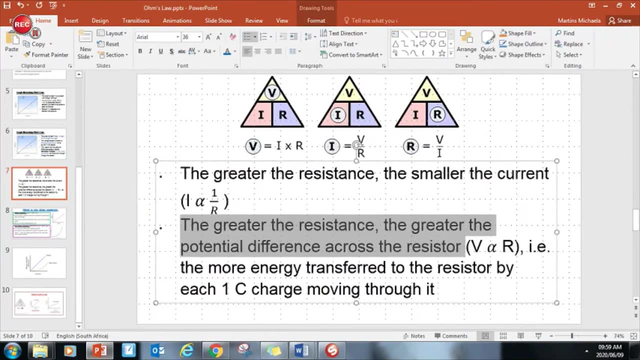 of the current, I'm going to have a smaller current. So it's like going back to this picture of this little resistance guy: If he provides more resistance, there's going to be less current flow. okay, the greater the resistance, the greater the potential difference across the resistor. 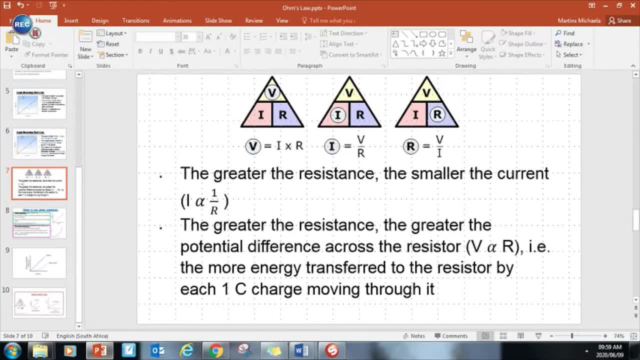 so what that means is, if i choose to include a resistor in my series and it has a very high resistance, i'm going to need to increase my potential difference because it's providing such a high resistance. in order to get my current to flow, i'm going to need a greater potential. 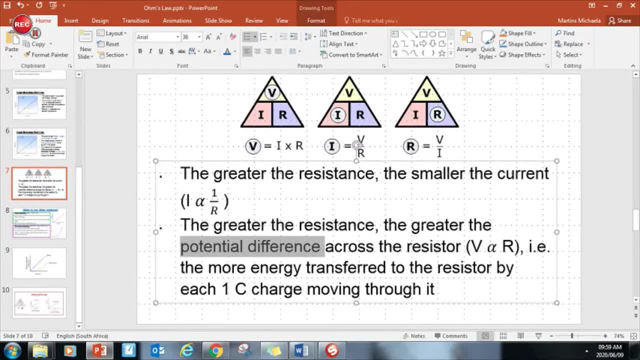 difference or a greater push. that makes sense. so v voltage or potential difference, is directly proportional to r. so you can see that here with this formula: if i increase r, so make this number bigger, v is going to go bigger. okay, now that just brings us to the last little section of this v. 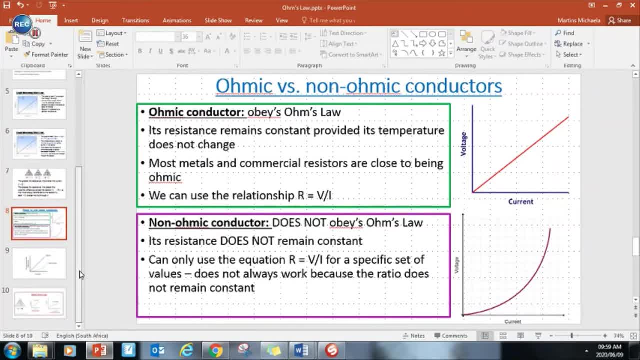 ohms law and you know what ohms law is. so if it obeys ohms law, we're going to see a straight line through the origin when i plot voltage and current against one another. so it means that the resistance is constant. the resistance does not change. here we can see straight line through the origin. 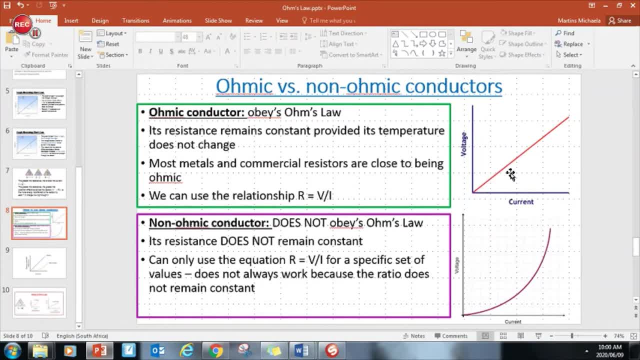 constant resistance voltage divided by current will always give me the same r value. so here, so we can use this relationship or this equation. and it says most metals and commercial resistors are close to being ohmic. okay, now, non-ohmic does not obey ohms law. look at this voltage and current graph. you do not see a straight line that 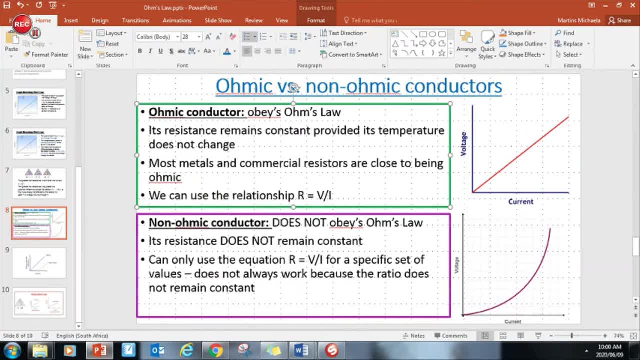 goes through the origin, you see a kind of a curved line. okay, so that means that the resistance is not constant. if i go voltage divided by current, i'm going to get different resistance values as i go along. so it'll only work. this equation will only work for specific values, for specific sets of. 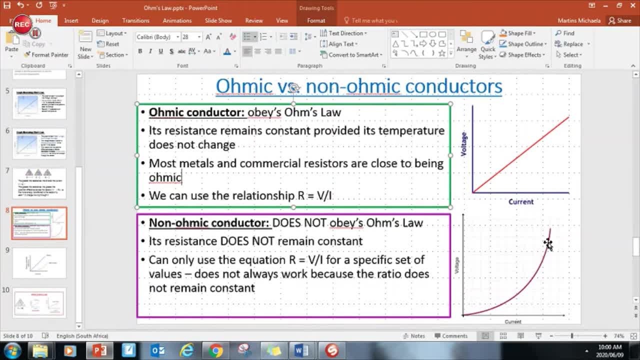 values. but it doesn't always work. the ratio doesn't always remain constant. therefore, resistance is not always constant. so you just need to be aware of how a ohmic graph looks versus a non-ohmic. here's another comparison. so this is voltage, or potential difference against current. here's an ohmic. 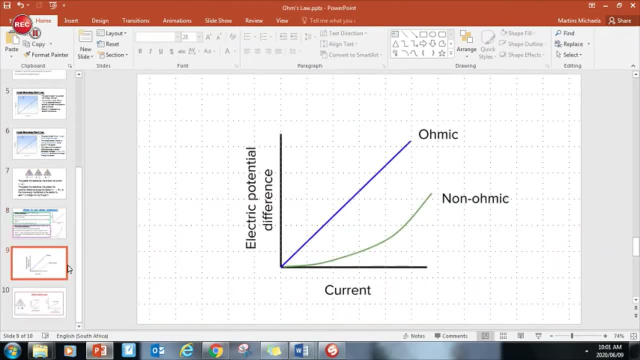 resistor and a non-ohmic. see it curves like that and again over here: resist resistance is constant here. if it's an ohmic, it's not constant. if it's a non-ohmic, it's not constant. if it's a non-ohmic. 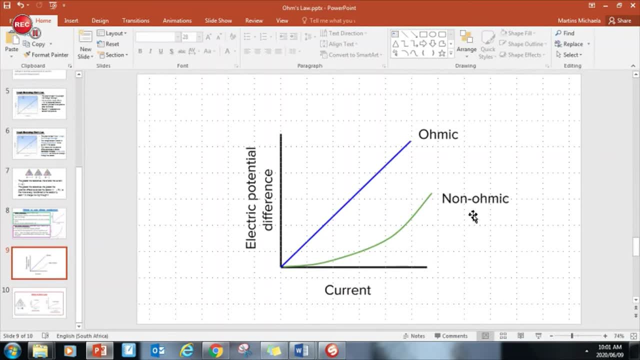 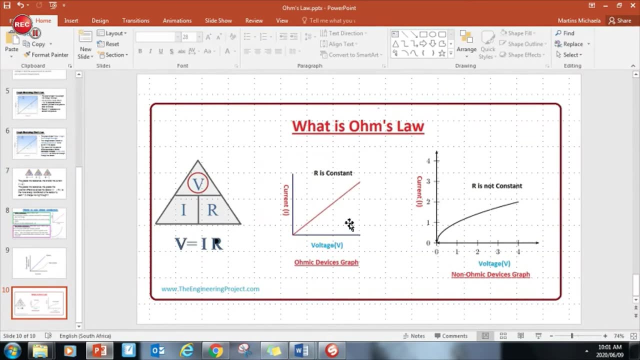 device. resistance is not constant here if it's a non-ohmic device. if you guys are paying attention, you'll actually notice that in this example they've swapped the axes. so here we've been doing- if you look at all these graphs, we've been doing voltage on the y, but if you look here voltage is. 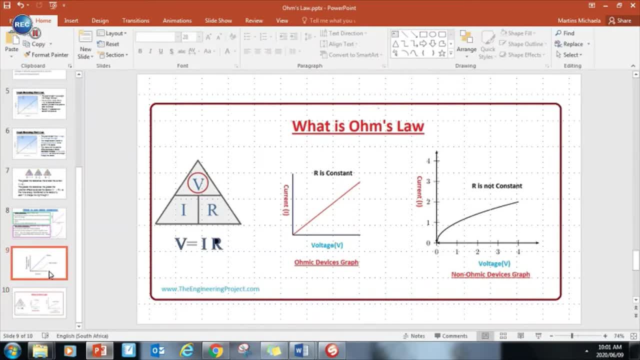 now on the x, that's okay, doesn't matter. all that means is that the gradient in this case won't be r, it won't be resistance, it'll be one over resistance. okay, it's not. it's not a massive train smash. say, you work out the gradient here and it's a half.